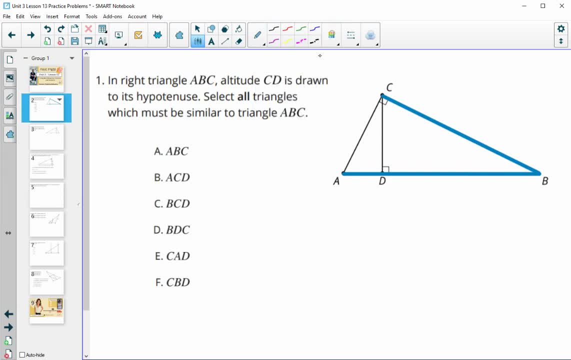 So when I'm going to compare this to the other triangles, I'm going to be making sure that it's going in that order that we're going to be going. we're going to be tracing the hypotenuse to the long leg and then finishing up on the short leg. 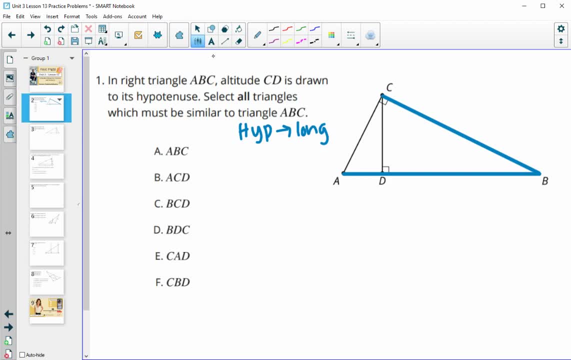 So, and hopefully I'll be able to show you that on the computer here. But all right. so triangle ABC, similar to triangle ABC. yes, anything is similar to itself by a scale factor. So we're going to go A, C, D and if we watch this, we're going hypotenuse to long leg, since this would be the triangle. 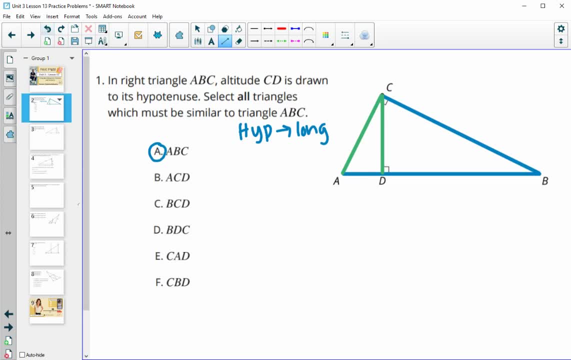 So hypotenuse to long leg. that's following the same order as the blue one, And so this one would be similar, since we're following the same order. So A, C, D. hypotenuse to long leg. Next one: B, C, D. 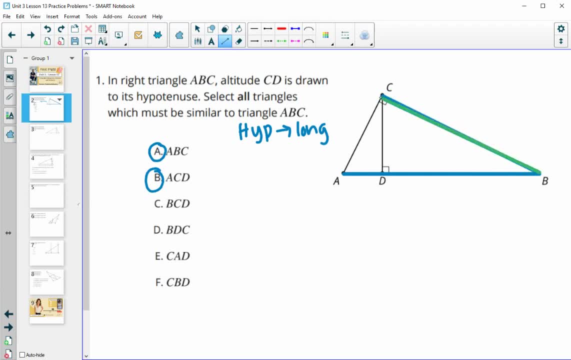 So we need to start at B, go to C and then D. So from this triangle here, if we're looking at this triangle, we went B, C, D, which is the hypotenuse, to the shorter leg. So this one is not going to be the correct order of segments. 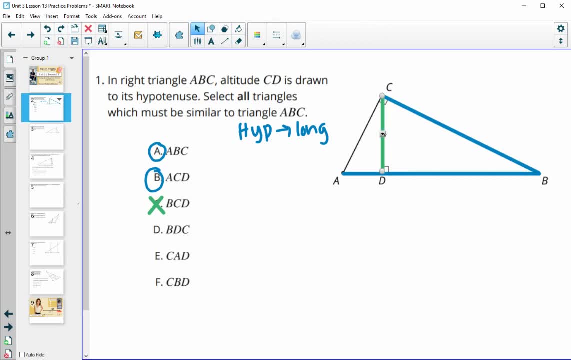 So that one is not going to be similar. Next one B D C. So B D C would be this triangle. So then we can see that we did the long leg and then the short leg. So this is not going in the same order because we would need to do hypotenuse to long leg. 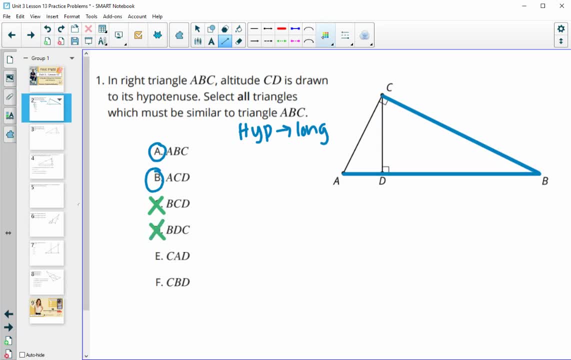 So long leg to short leg, not the correct order. Triangle C A, D, So C A and then D. So in this one we went hypotenuse and then short leg, finishing up on the long leg. So that's not correct. 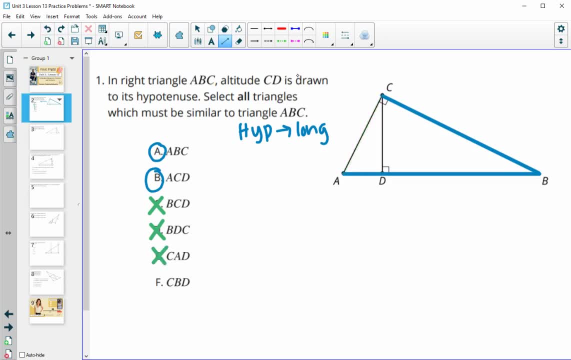 We need hypotenuse to long leg. And then last problem, or last triangle, says triangle C, B, D, And so that would be this triangle, And we did go hypotenuse to the longer of the two legs, So this one would be true. 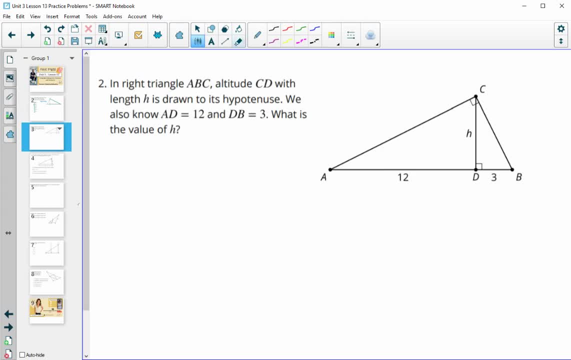 Number two in the right triangle, ABC, we've got the altitude drawn down to the hypotenuse, So CD, here is our altitude. And then we want to find the value of H, knowing that AD is 12 and BD is 3.. 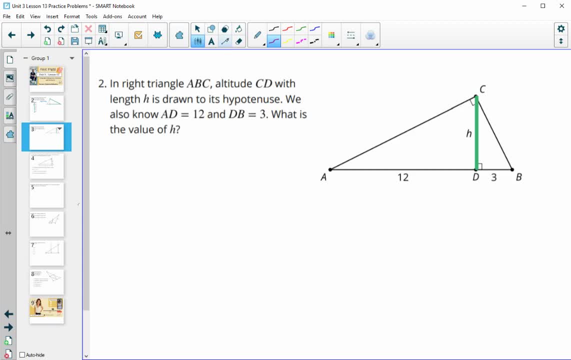 So we know that when we take kind of these two triangles separately here, So we've got this triangle, That's the long leg and the short leg in this purple triangle, And then in this green triangle we've got CD as our long leg and then BD as our short leg. 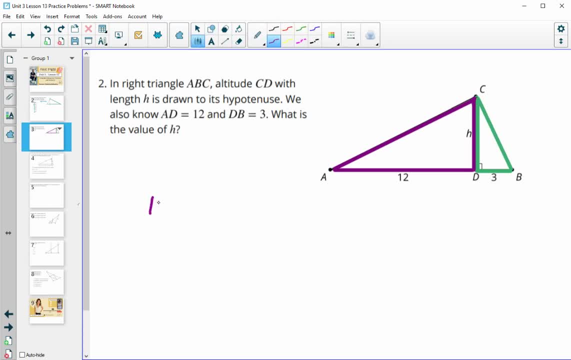 And so we can kind of set up a proportion here. So if we take the long leg and the purple divided by the short leg, that's going to equal the long leg in the green triangle, which is H, divided by the short leg, which is 3.. 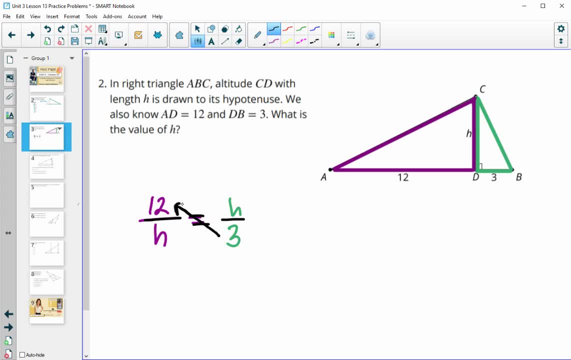 And then we can cross, multiply and solve this proportion. So we've got 3 times 12, which is 36.. And H times H, which is H squared Square root both sides, and we get that 6 equals H And H times 1 equals 3.. 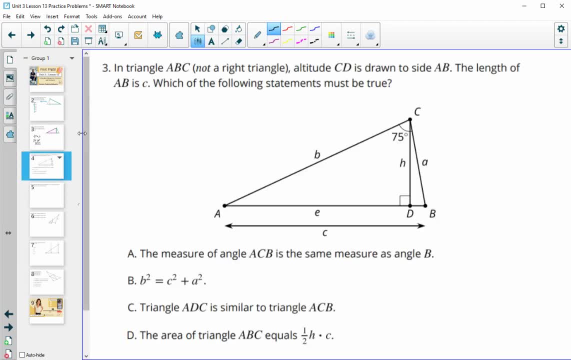 So we're going to have to add that into our式. So look, watch this and make sure that you're paying attention. All right, Number three In this triangle ABC, which is not a right triangle. Okay, so triangle ABC is not a right triangle. 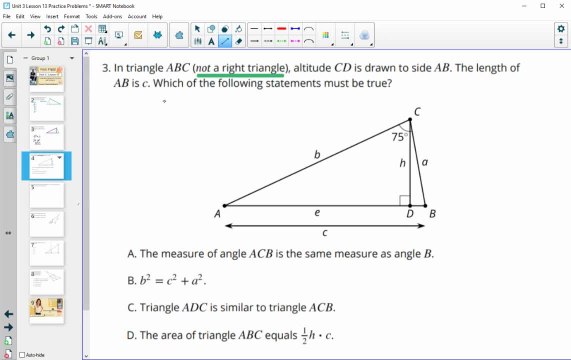 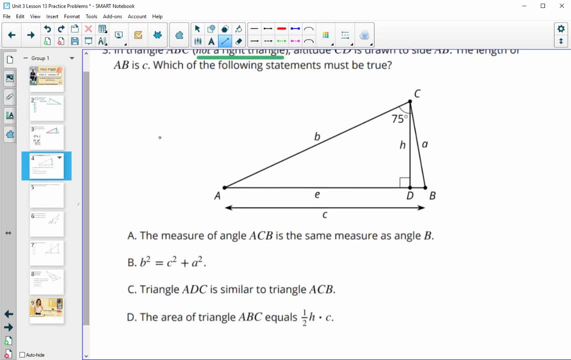 We do have the altitude drawn to the side. The length of AB is C, So this long side down here is C. Okay, so now we don't necessarily know that we have similar triangles because we don't have a right triangle here. so in order for all of these triangles to be similar, the altitude has to. 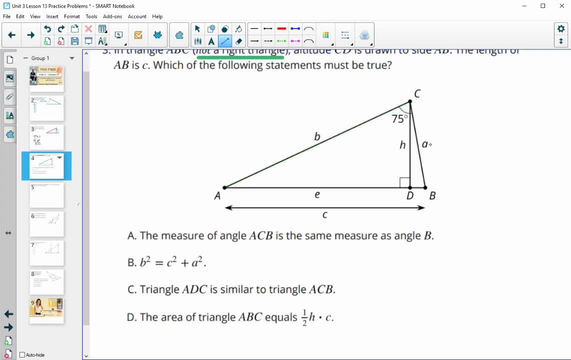 be drawn from a right angle. so we don't know that these three different triangles are similar. therefore, we don't know anything about their angles being the same. so angle a, c, b- we do not know if that's the same as angle b here. um, this green triangle here has side lengths of a, b and c. 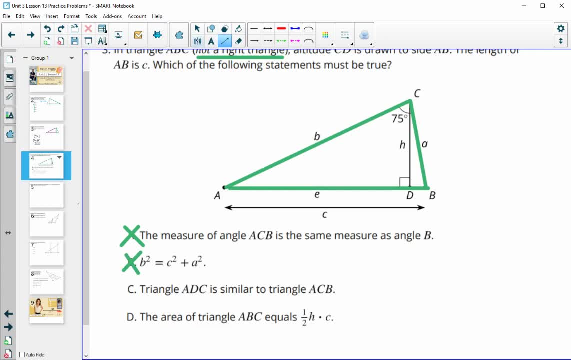 but we would not know that we could do pythagorean theorem here, or pythagorean theorem wouldn't work here because it's not a right triangle: um triangle a d c, um triangle a d c, um triangle a d c. so let me get that. so triangle a d c is similar to um triangle a c, b and we're not going to know. 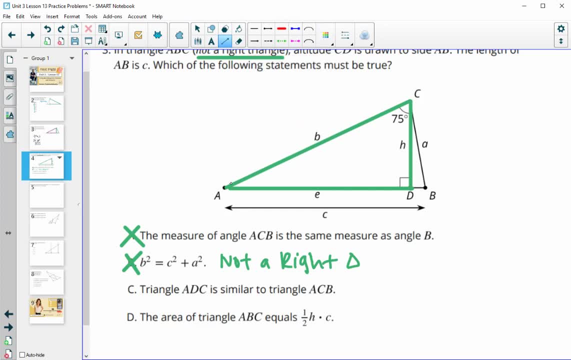 this because we don't have the right triangle to begin with um, but let's draw it anyways. so a, c, b, okay, again um. nothing to tell us that those are going to be similar, since we don't have two matching angles and we're not drawn from a right triangle. 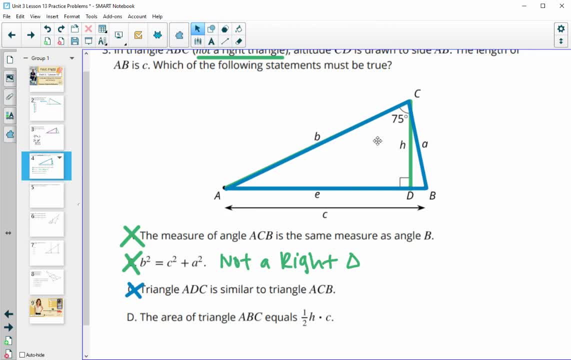 and then finally, um. the area of the green triangle equals h, which is this hype, um, this altitude here, okay, equals h times um c divided by two. that is true because h the altitude is your height and the c is your base, and we can see that those meet to form a right angle and area of a triangle is one half base times. 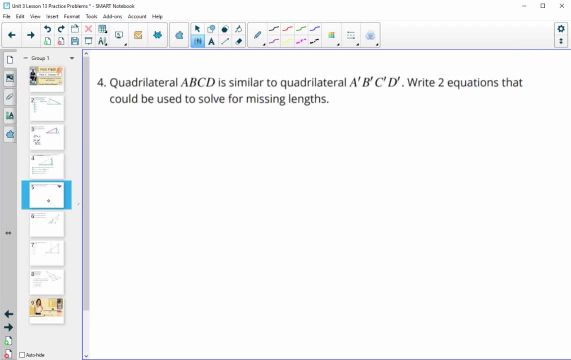 height. so this one is true. number four, quadrilateral: a, b, c is similar to a. prime b, prime c, prime right, two equations that could be used um to solve for missing lengths. there's gonna be tons of equations that would be correct here, um. so let me just set up a couple proportions so i could. if i knew um ab, i could do. 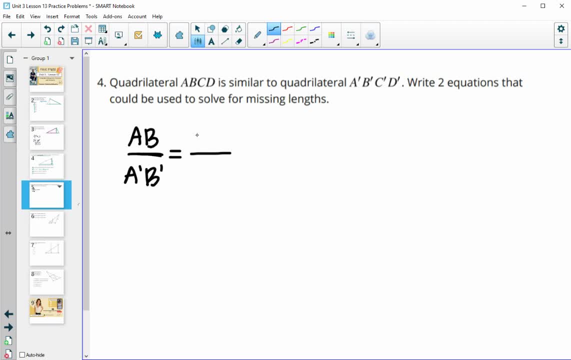 ab over a prime b prime and then set that up with any other corresponding sides, so b: c over b prime c prime. this could have been cd over c prime d prime. these could be flipped over so i could have like a prime d prime over a, d equals b prime, c prime over bc. you could do um. 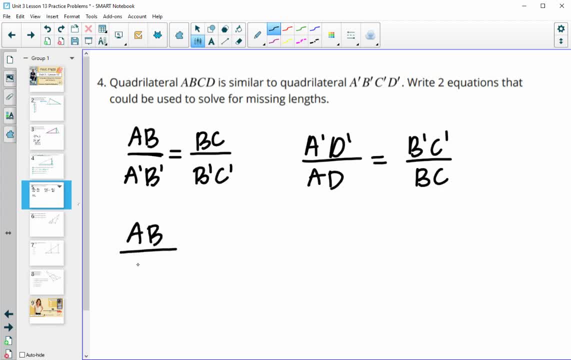 original. so i could do like a b over um a d and then that would equal the prime version of those or image version of those. so you could do a ton of different proportions. I would argue you can also say that the new length or the image is equal to the. 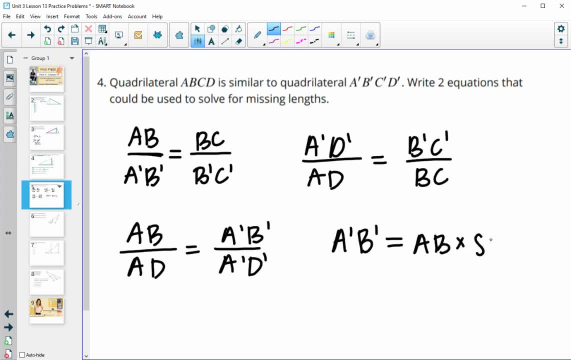 original times the scale factor. so make sure you know what that means, but scale factor. or you could also find the original length by taking your image length divided by the scale factor. so I'd argue you could even do something like that, but there's a lot, a lot, a lot of different answers that would work. 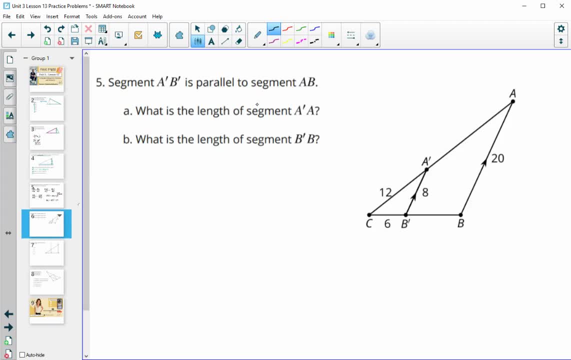 here number five, segment a- prime B is parallel to segment a- B. this means that we've got the proportional sides and we've got the proportional sides and we've got the proportional sides and we've got two similar triangles. so this one wants to know what is the length of a prime B? 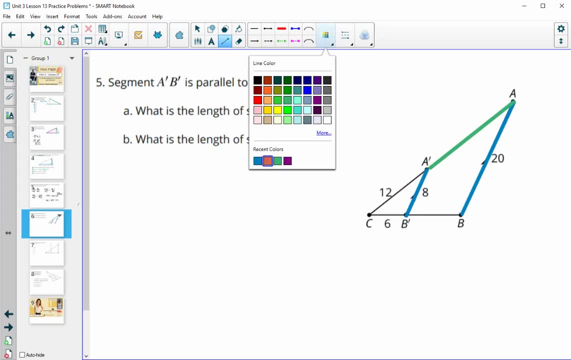 or sorry, a prime a, and also what is the length of B prime B. so these are just portions of the sides, but we don't have either of them, so we're not going to be able to say what the what the factor is from twelve to this side or six to this. 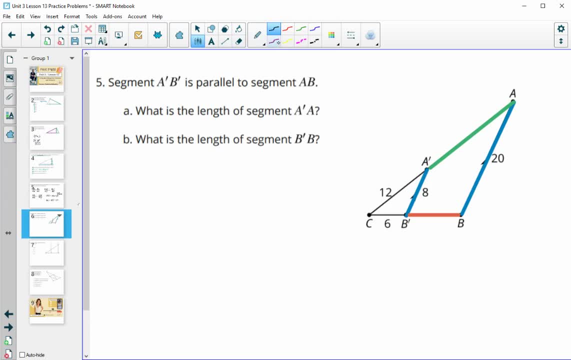 side right now. so we're gonna want to look at the actual triangles here to get the scale factor, and so let me draw in these actual similar triangles for a second. so we've got this large triangle here, similar to this smaller triangle here, so let's just solve for those large green lengths and 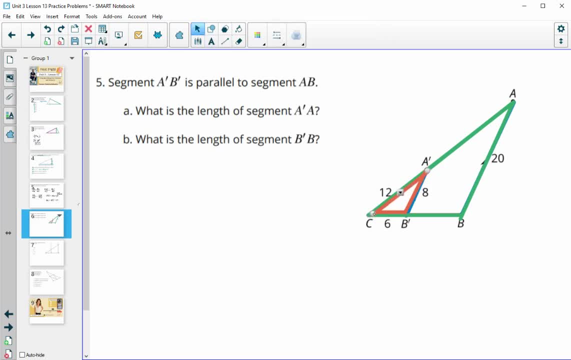 we'll be able to figure out the missing parts of them. so if we take a look here, we see that we have kind of the base of each of these. are this parallel line part of each of these? and so if we look at what the scale factor is here, the scale factor is twenty divided by eight. 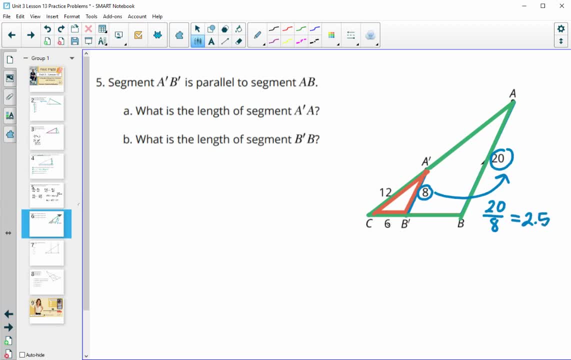 which is two point five. so now we know, if we take C, B, prime, times the scale factor, so times that two, it's this we can say까요 these are the two pieces 2.5, then we'll be able to get the length of BC. So 6 times 2.5 is 15.. So I know that this whole 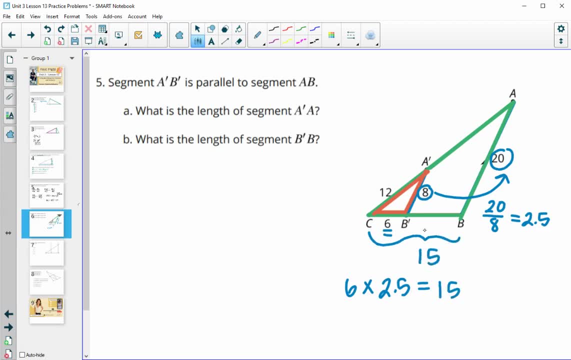 side here is 15.. So then if I want this little piece here, I would just do 15 minus 6 and get 9 for this part. So this piece here is 9.. So that's the answer to part B, And then, if we do, 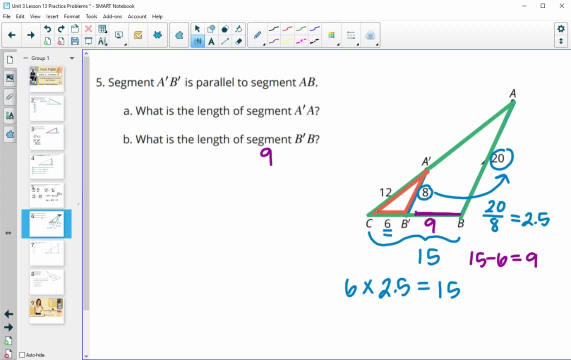 a similar idea here. we know this: A prime C is 12.. So we can take a look to get this, And so we can do 12 times 2.5, which gives us 30.. So 30 for that whole thing. And so then this piece here is: 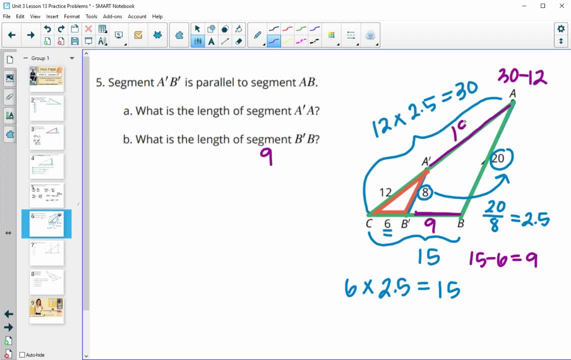 just going to be 12 times 2.5.. So that's the answer to part B. And then, if we do a similar idea here, we know this A prime is going to be 30 minus the 12 we've already used. So A prime is: 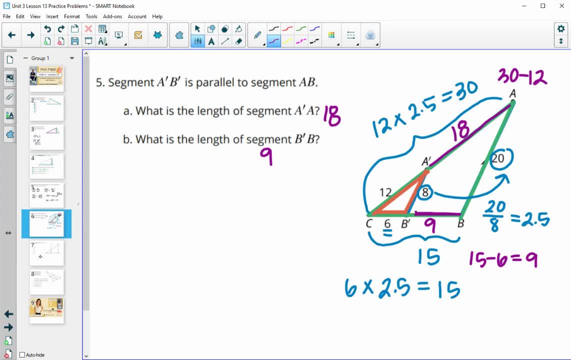 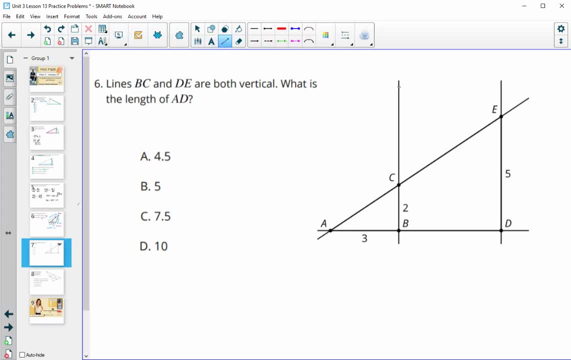 going to be 18.. All right. number six gives us two vertical lines, BC and DE, And since they're both vertical, we know that they're parallel to each other. So we're splitting, we're getting proportional side splits and we're getting proportional triangles, So we want to find the 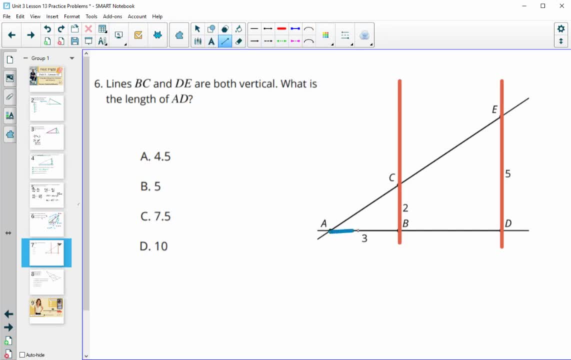 length of A prime. So we're going to take a look at that. And then if we do a similar idea here- AD in this case- so we want this whole length here. So we're kind of looking at this larger triangle. then, if we want the whole length of AD versus this smaller triangle here, 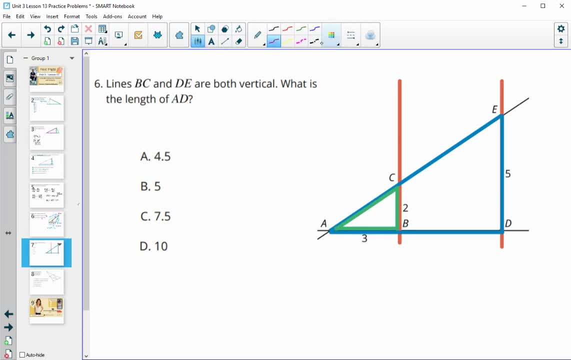 So we see that we have the two and the five. So we can look at the scale factor. that takes two to five, And so two times 2.5.. You can also figure that out by taking the five divided by two. So then we could take this three. 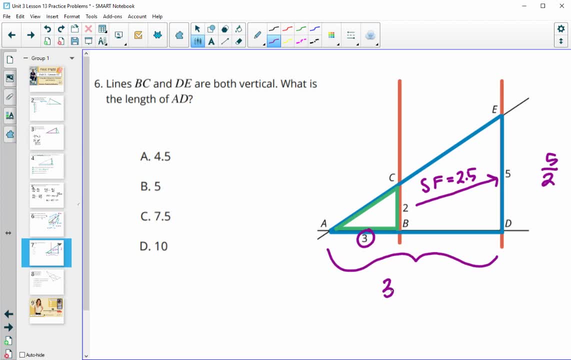 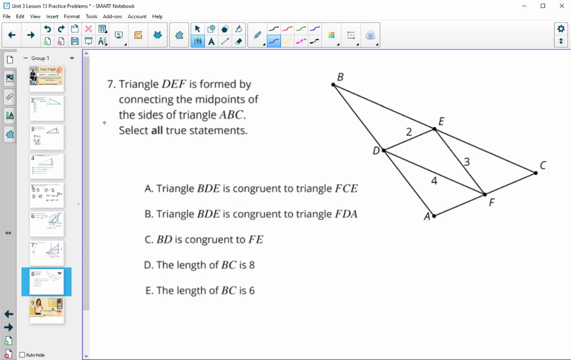 to get this side length of AD. So three times 2.5 is going to give us 7.5 for AD, And then that's what we wanted was the length of AD, So 7.5.. All right then. number seven says triangle DEF is formed by connecting the midpoints of the sides. 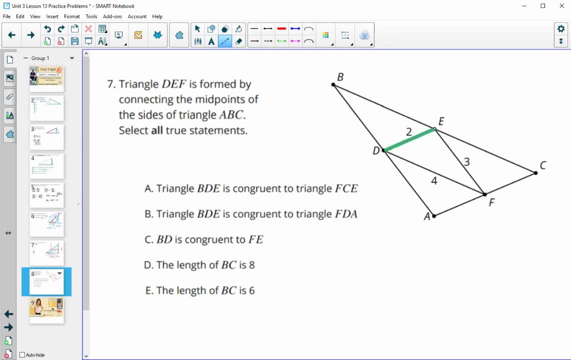 of the triangle, When that happens, when we connect all the midpoints. all these little triangles here are congruent to each other, just from a rotation of this inner one, and then translation, So kind of the ones that are not highlighted in green are translations of each. 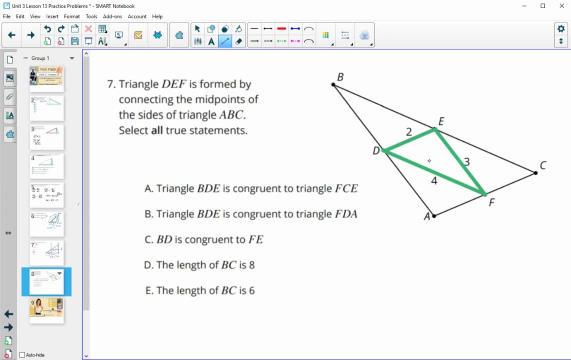 other, And then this middle one is going to be the middle one, And then the middle one is going to be the middle one, And then the middle one is a rotation. So when we're looking at if they're congruent, we got to make sure that we look at the order in which they name the sides. So this: 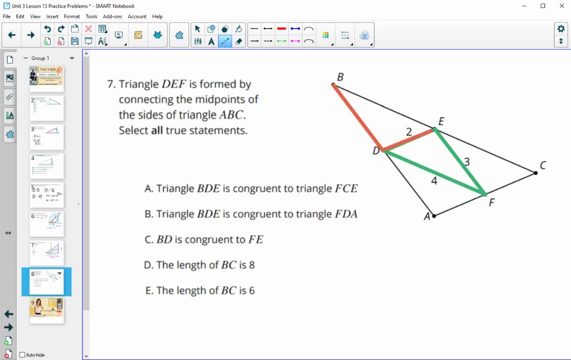 first one says triangle BDE. So here's the order that we went in BDE, And then it would close up here. But I'm just going to not do that So we can compare to the next one. So then, triangle FCE. 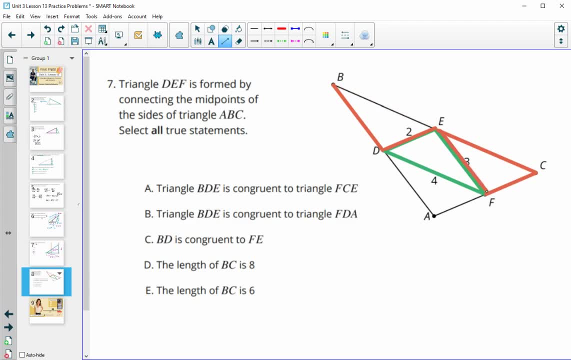 E. We can see that it didn't go in the same order, since it went to this small angle first. So this is not true. The two triangles are congruent, but we have to write the order of the letters the same. So BDE is not congruent to FCE. 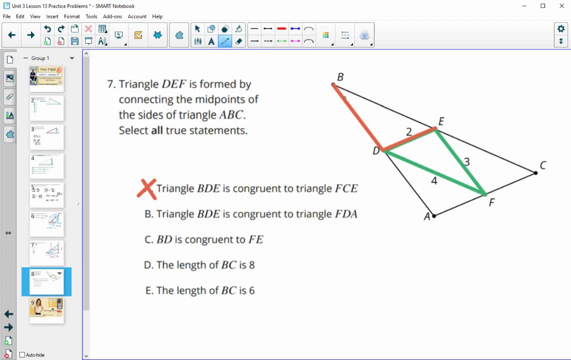 If we went in the same order it would be So if we had done BDE to EFC, that would be fine, But the order that they did it not true? Next one: they still did BDE And now they went FDA. 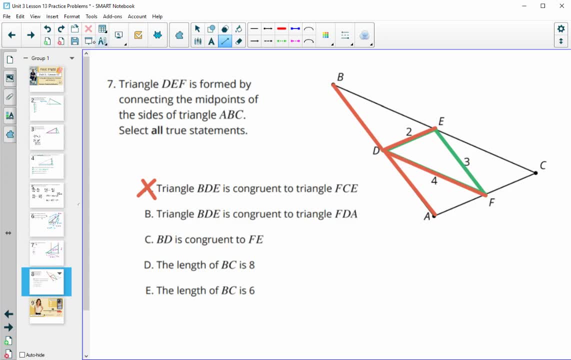 So again not in the correct order, since that went to that small angle first. So this is not true either. They're not matching up the corresponding parts correctly, All right. Then C says that BD is congruent to FCE. So that's wrong. So that's wrong, That's wrong, That's wrong, That's.